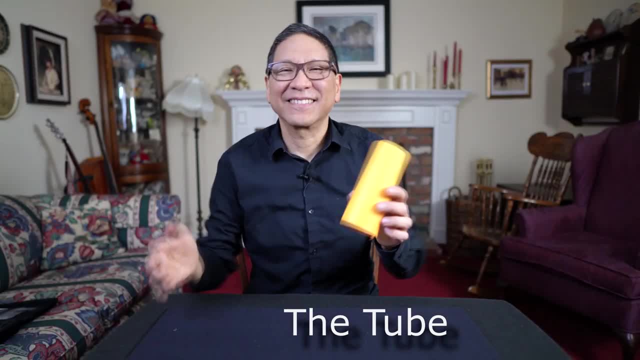 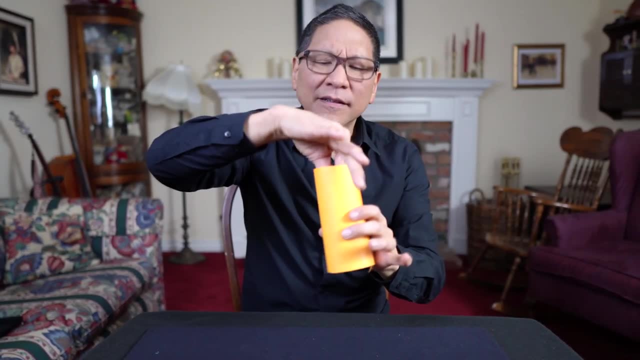 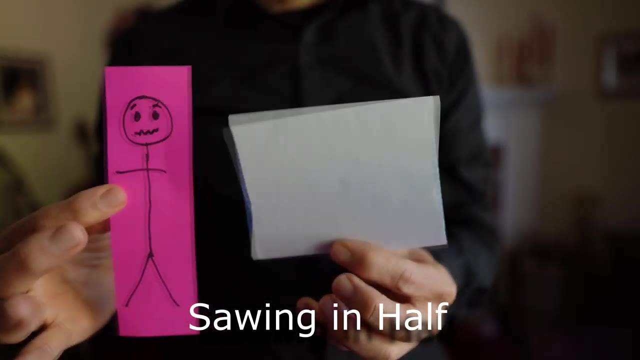 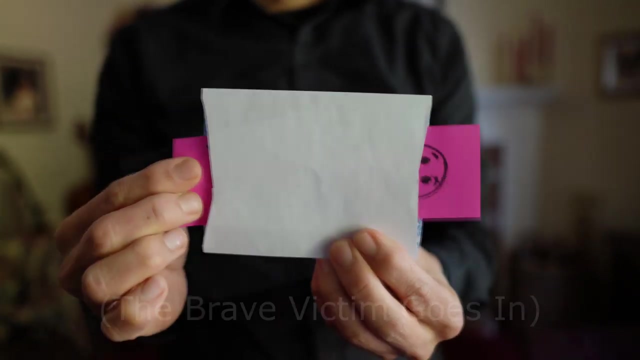 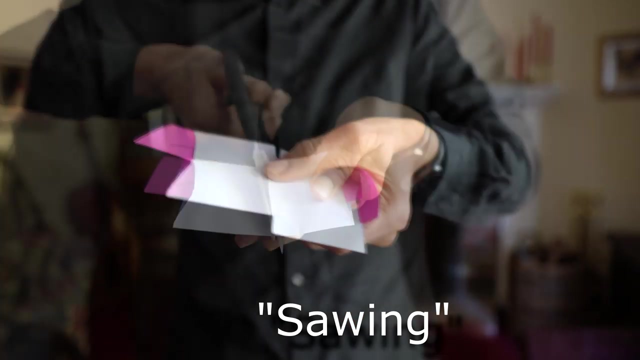 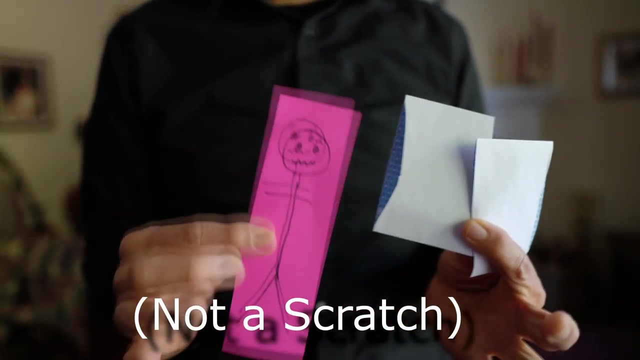 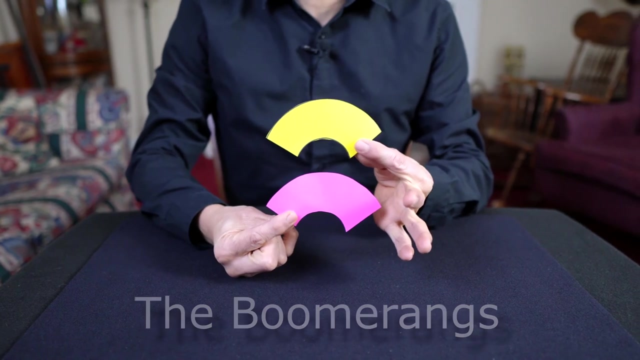 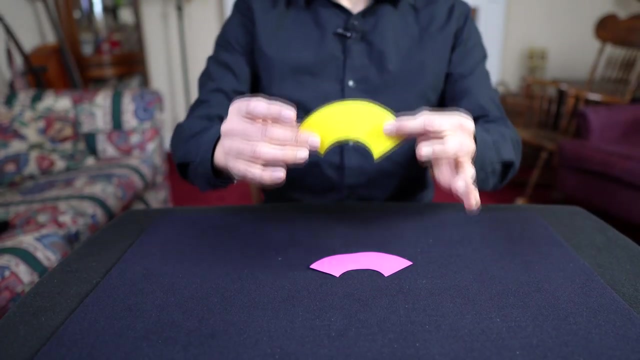 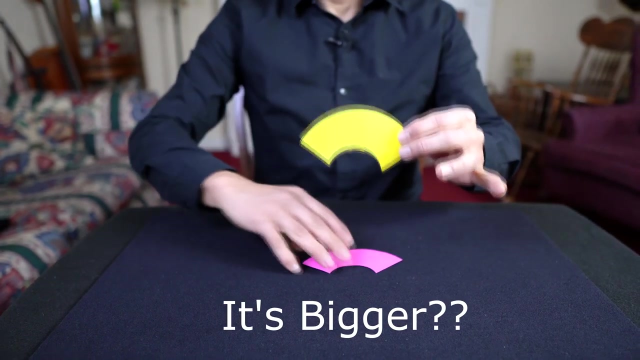 Come on. Come on, two boomerangs here and you notice that the pink one is larger than the other one. let's do a little magic spell here. they just snap the finger. we're gonna cause this yellow one to increase in size. and if I've been successful, check. 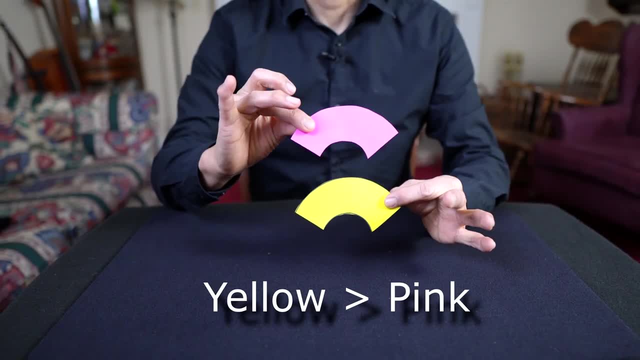 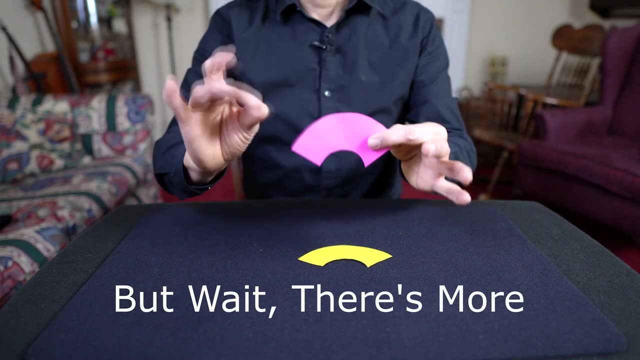 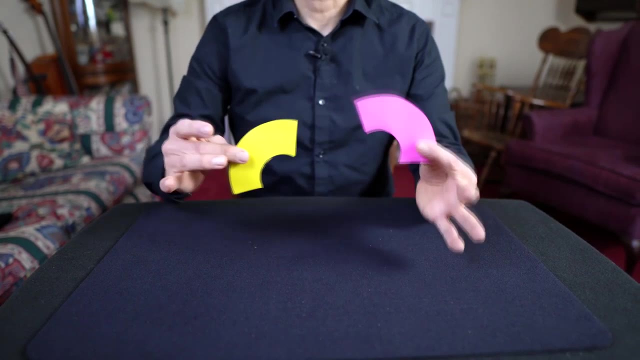 it out. I think that worked. the yellow one is now bigger than the pink one. but wait, there's one more thing I can do. if I just cause a little bit of a minor spell here, if I snap the finger will enlarge the pink one just a little bit. 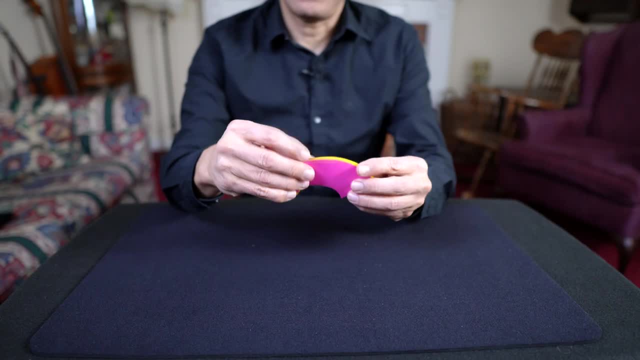 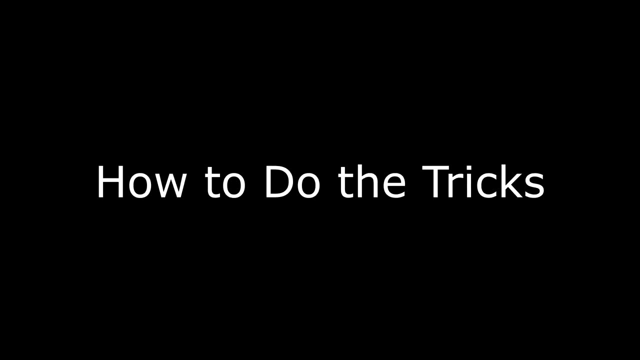 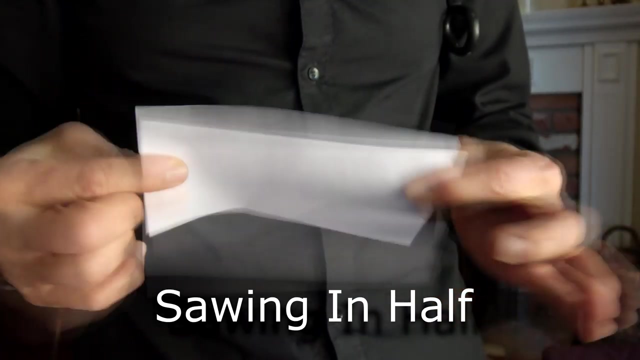 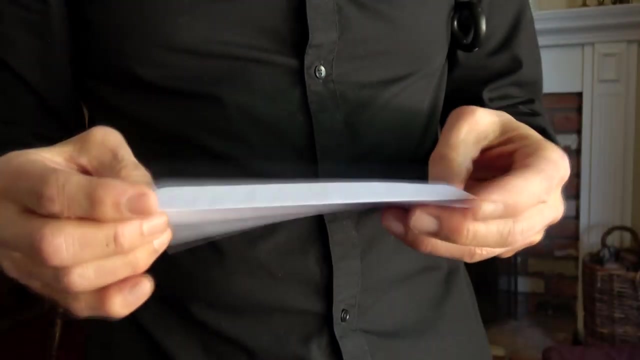 and you'll now notice that they are the same size. here's how to make your gimmicked envelope so you can perform the cut and restore effect. take your envelope, just an ordinary envelope. it could be pretty much any size because you can cut it down to the size you need, depending on 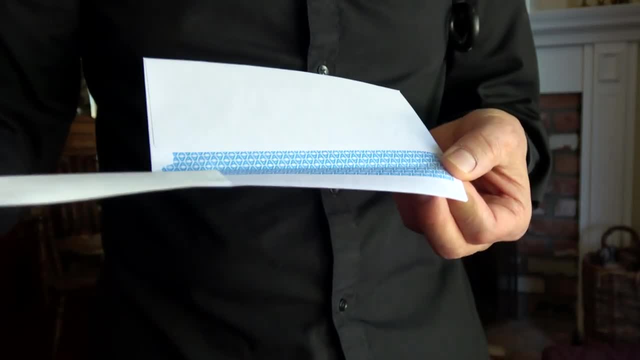 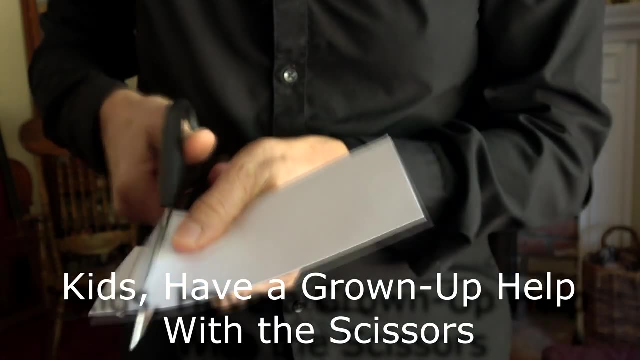 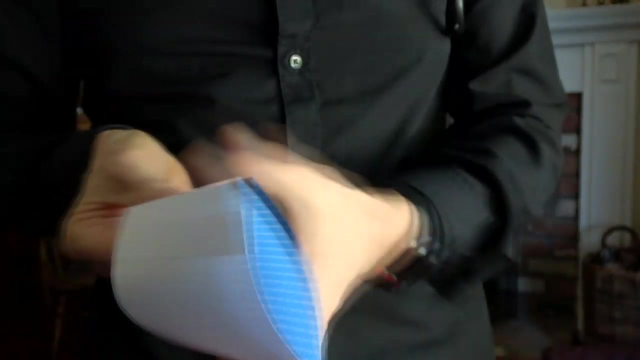 what it is. you're going to cut in half, or apparently cut in half. seal the envelope first. now take some scissors. you're going to cut the end of the envelope and you're going to cut the end of the envelope off. what you end up with is a tube made out of an envelope. now, it's nice to have. 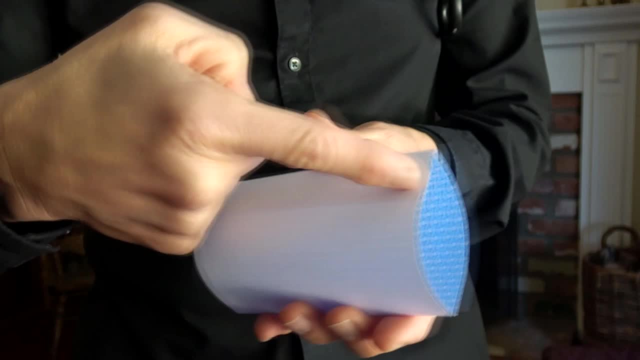 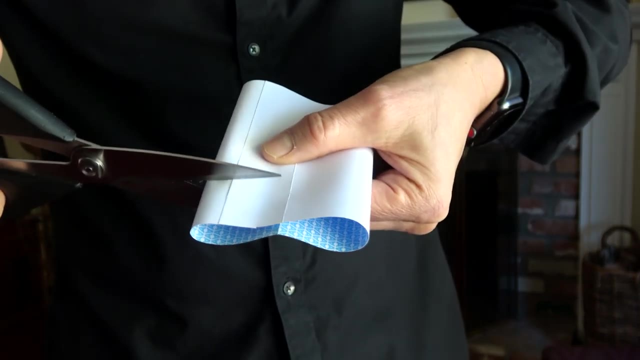 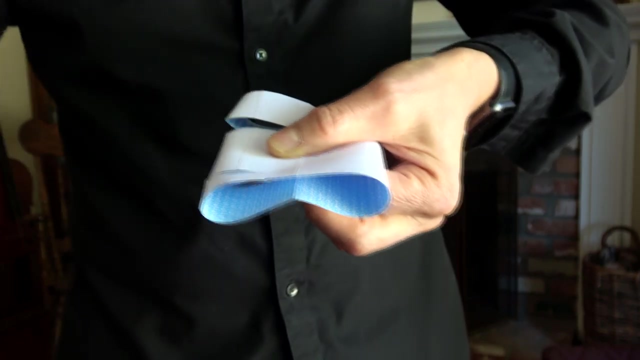 the clean front towards the spectators, are going to give me the back, the parts that has the flap, the sealed flap. going to take your scissors and you're just going to cut a couple of slits here. don't go all the way, but just go pretty much the full height. 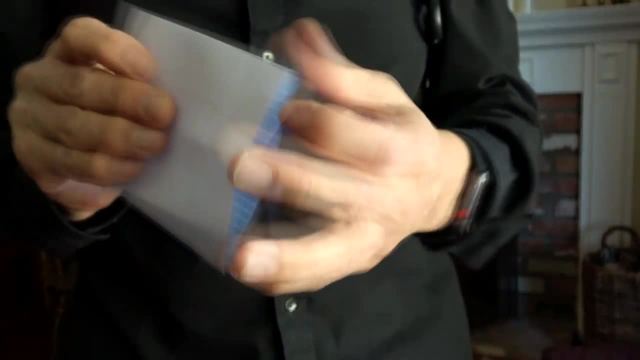 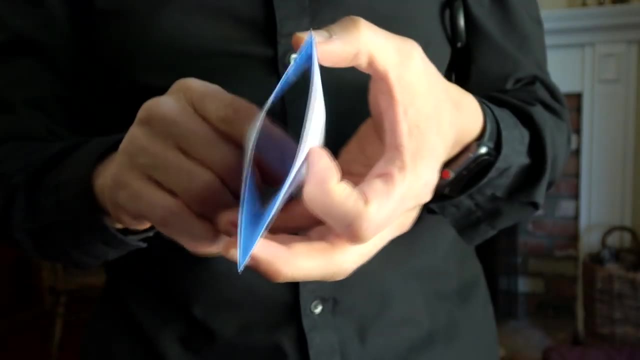 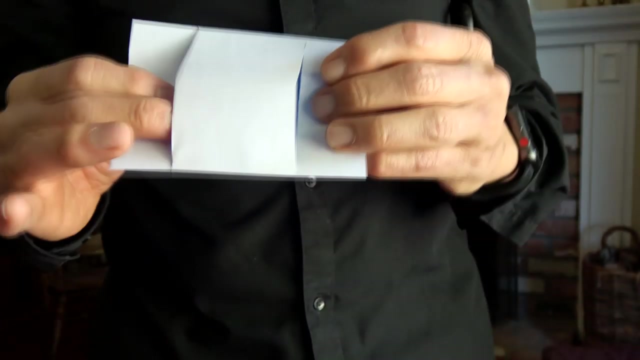 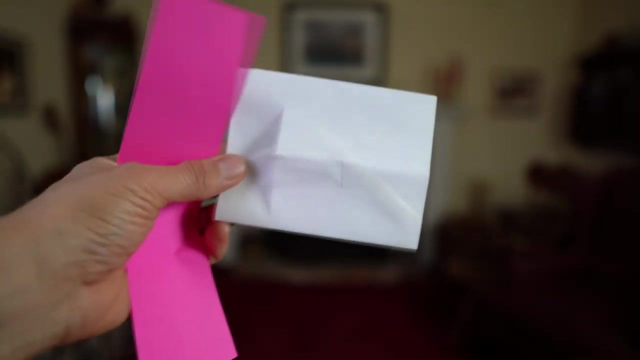 of the envelope and then, when you push them back together, you end up with a tube that has two slits in it. It's a secret to the trick. Now let's talk about how you can perform the trick with your gimmicked envelope. You have your envelope in hand. You have the slit. 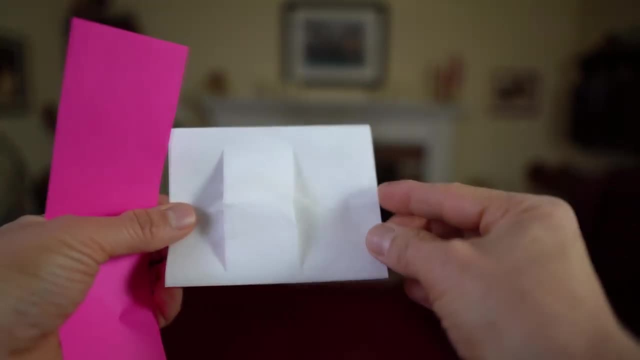 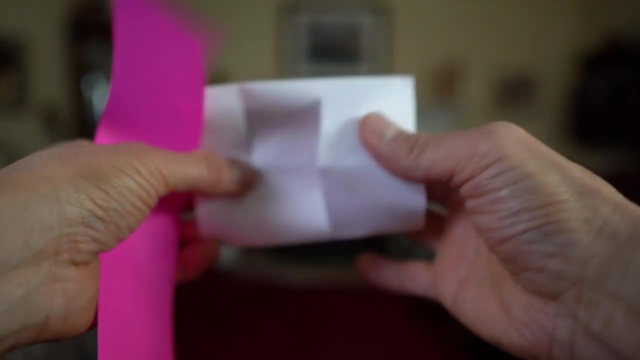 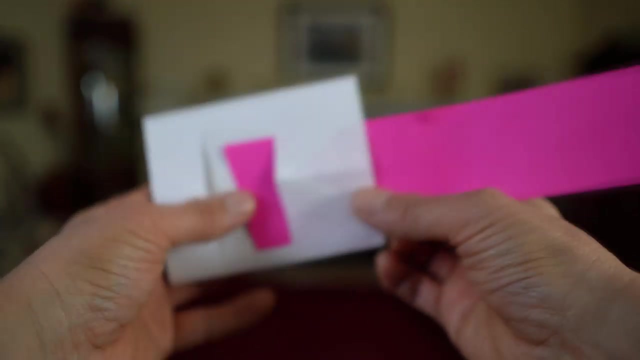 right there in your envelope and, of course, as we showed you in the construction, you have the tube. So here's how you perform the trick. Take whatever object you're using. We're just using a piece of paper here, but you feed the object inside of the envelope, as you can see, right there, and the 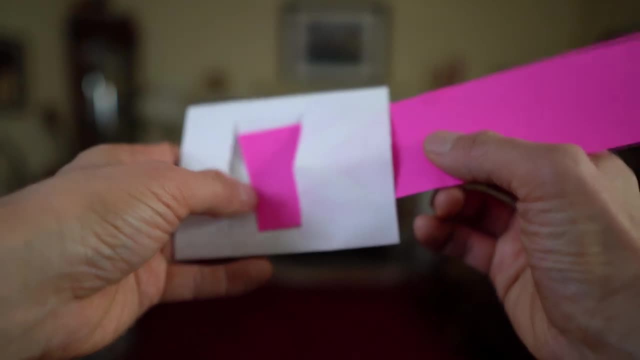 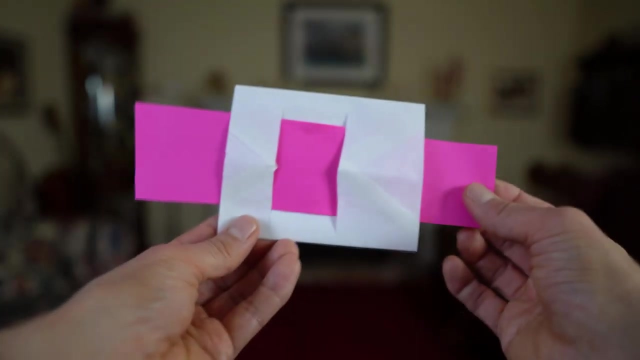 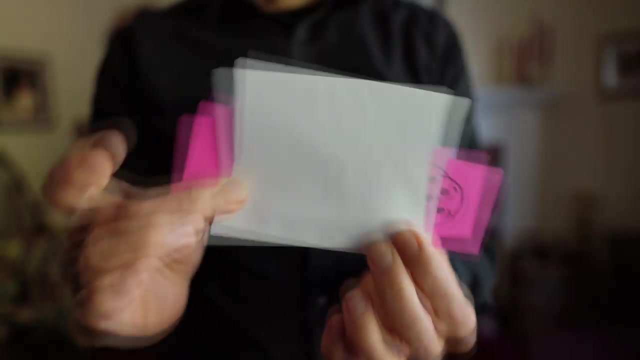 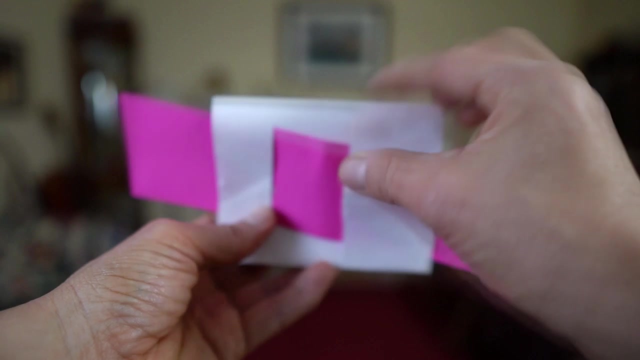 spectator's view, would be here Feeding the envelope through and then feeding it through the other slit there. And now the paper from the other side looks just like it's passed through the envelope tube, But what you've done is actually slipped it out the back, and therein lies the secret. Now you're ready to perform the cut. 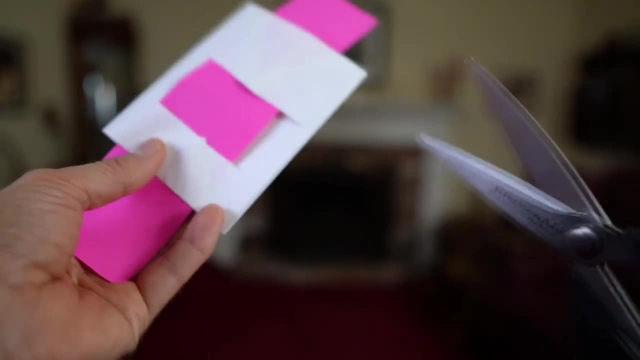 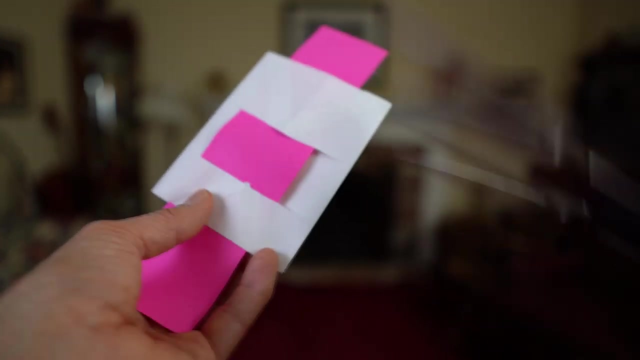 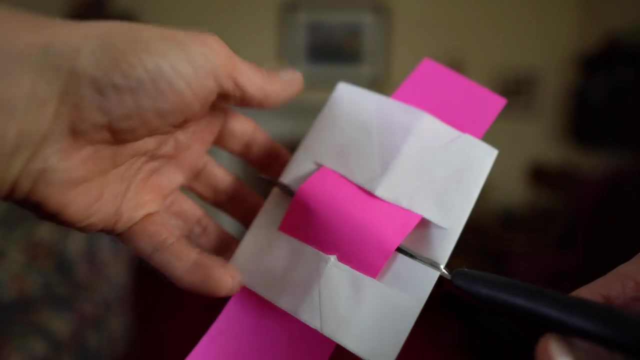 Remember, don't turn it like this and show the spectator. You don't want them to see the back, But you take your scissors and now the scissors go underneath, whatever the object is, whether it's a bill or playing card, And you cut with the scissors and from the front it looks as if you're cutting through. 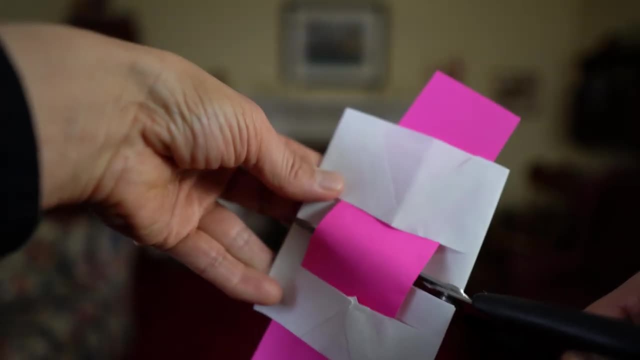 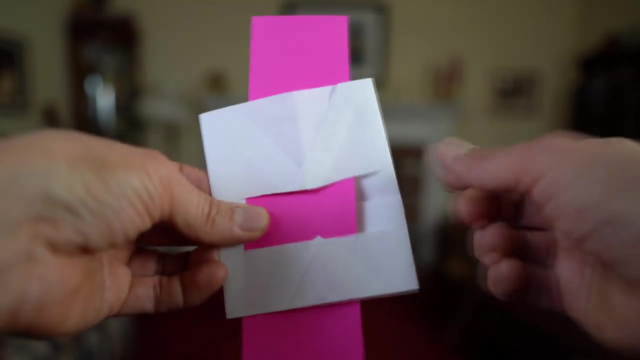 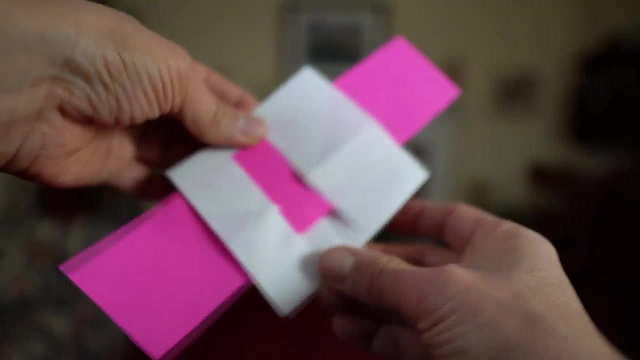 whatever's insideight. Now it helps to hold everything here so it doesn't come apart. Move the scissors. You've obviously clearly cut through. I like to hold it just for a moment So spectators can let that sink in that somehow you've cut the object in half, the envelope. 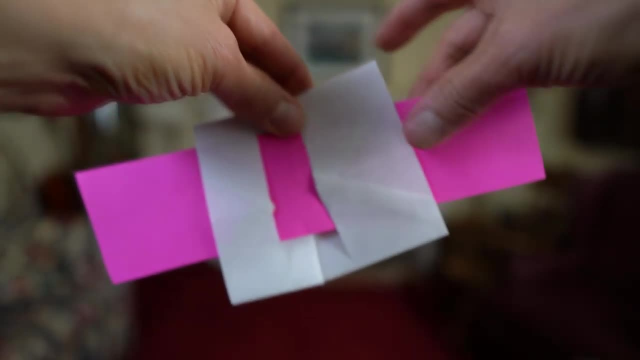 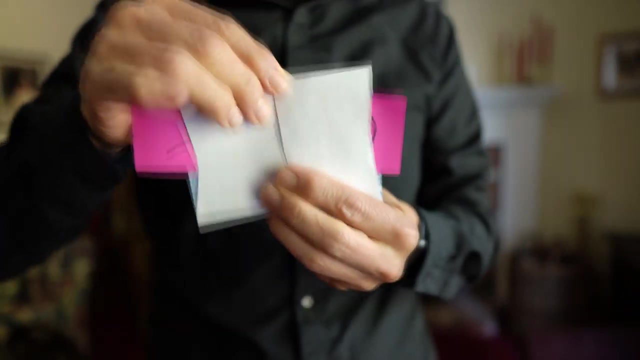 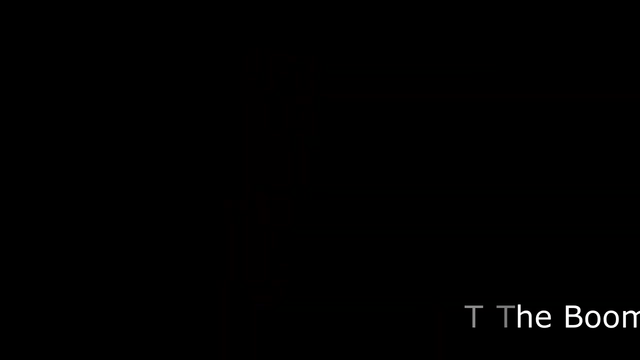 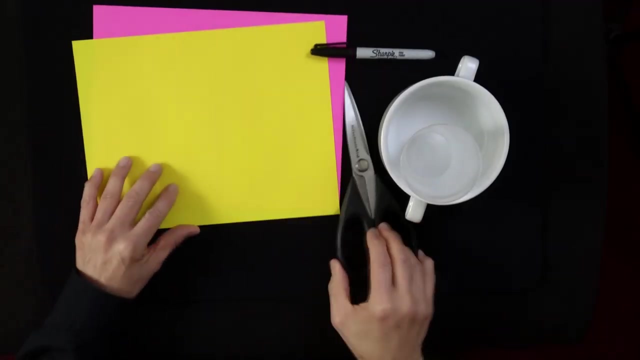 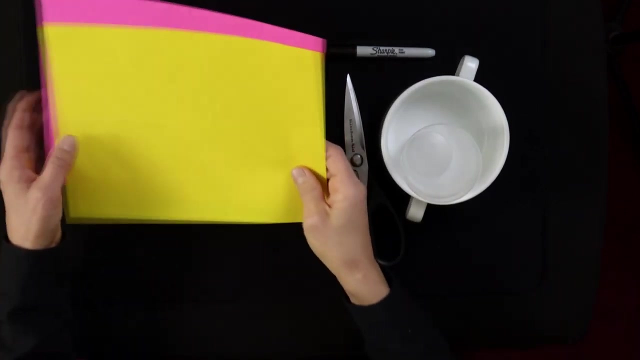 or tube and the object in general side, but then you can remove it and show that it's whole, and that's how you perform the cut and restore. here's what you'll need for the trick. you'll need two sheets of paper. helps to have different color papers and you can use the same colors for the boomerangs. 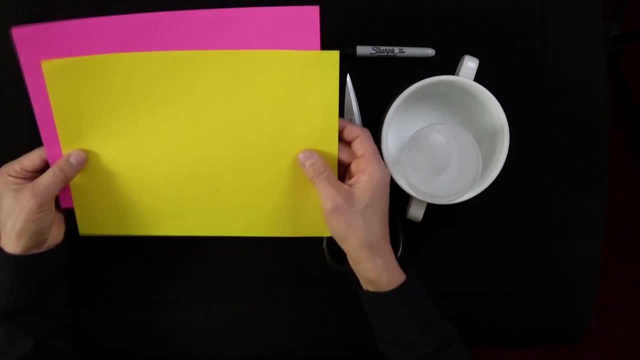 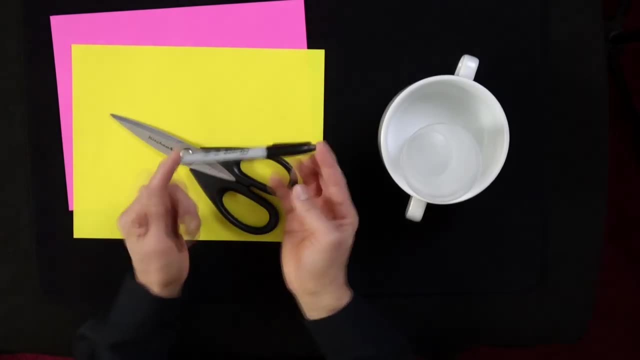 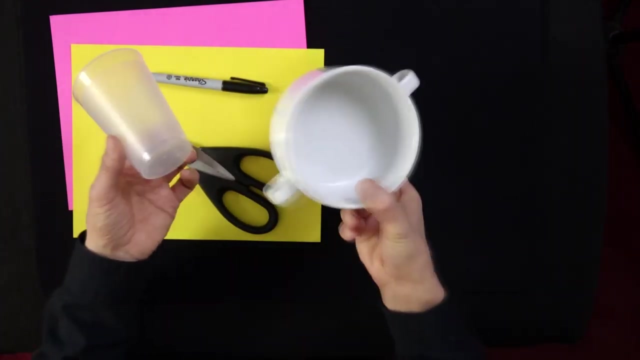 but you'll probably want to label them, so there's a little bit different about them. for the trick itself, you'll need a pair of scissors, you'll want some type of pen or something to mark with. and what are these this? what's the cup in the soup mug for? well, this is so you can actually create your own boomerangs. 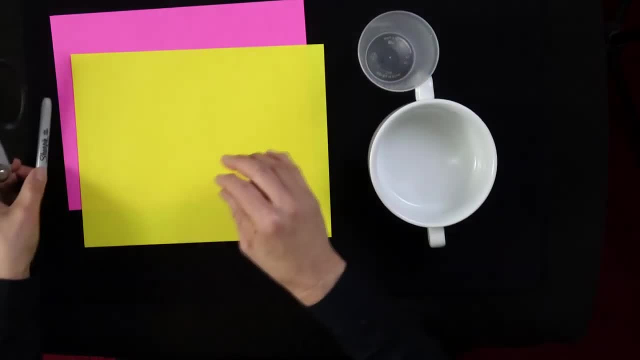 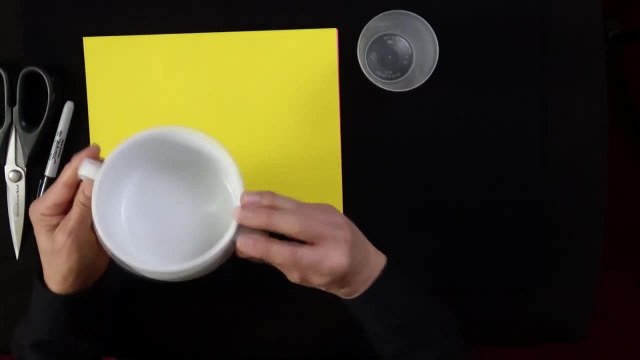 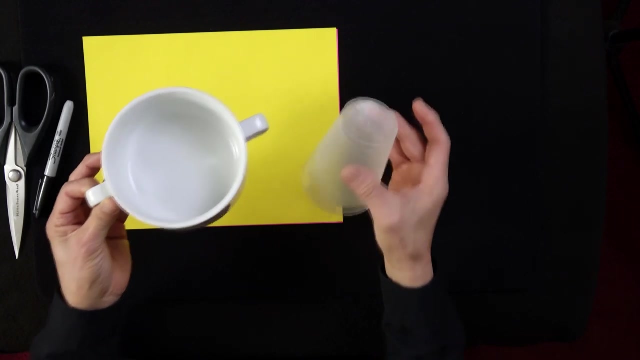 so let me show you how to do that. so let's set this aside for now. take your two sheets of paper, line them up. what you're gonna do is take your. you have to go through the house and look for circles with bowls, plates, cups, whatever you have. I've chosen these two because what I want are two different. 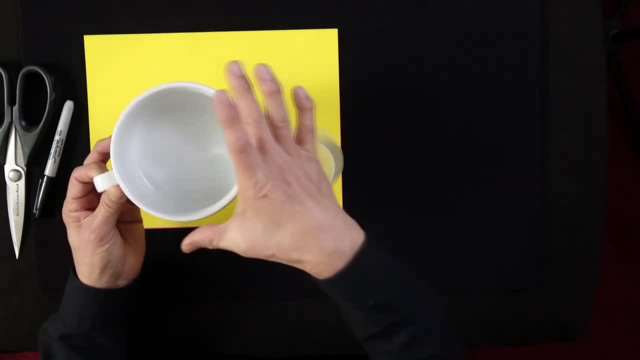 diameters is a diameter here and a diameter here. so one, the larger diameter object's gonna create the outer diameter of the room and it's going to create the outer dimension, Euclid, by the way, and that's going to create the outer dimension, Euclid, by the way. 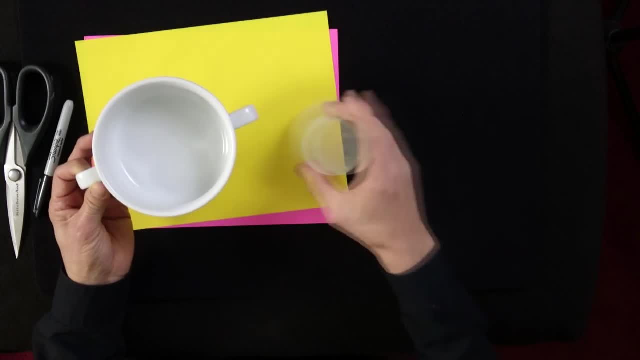 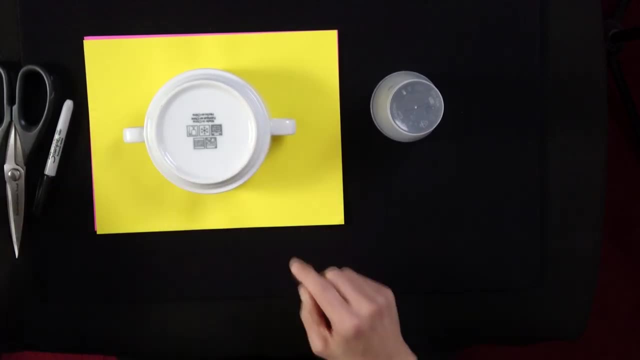 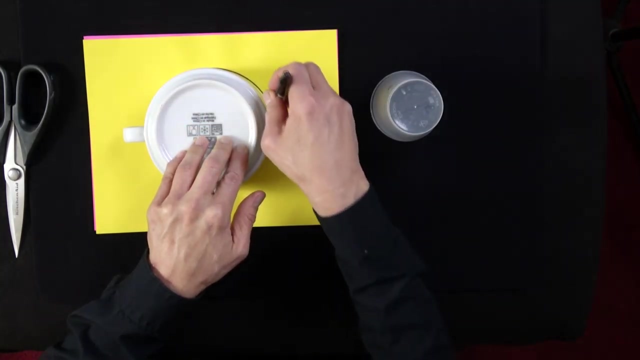 diameter, the smaller one will create the inside diameter. so let me show you how that works. I'm going to take this, place it down, I'm going to trace along the edge. all I need is a semicircle, so let's just do that, and I have a semicircle now with. 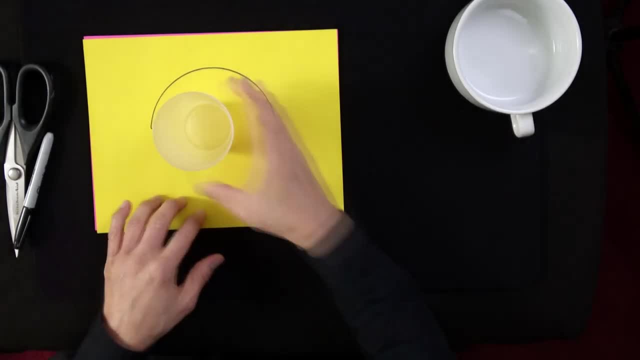 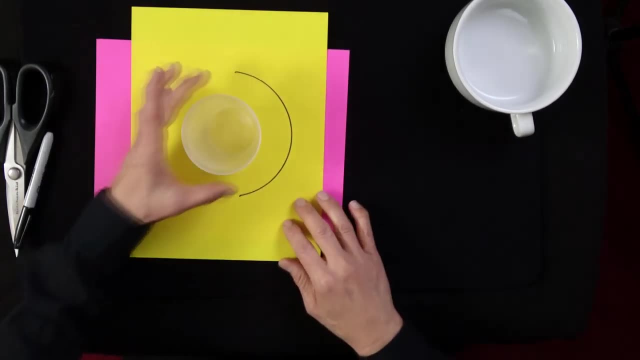 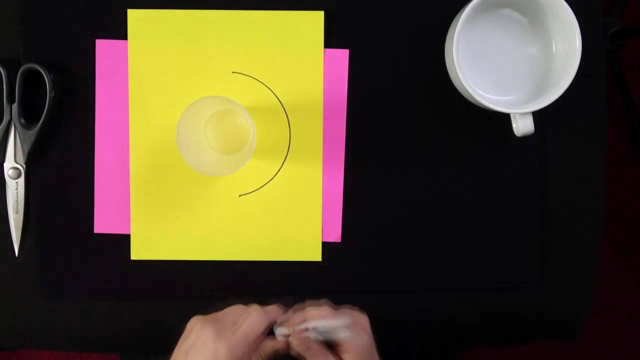 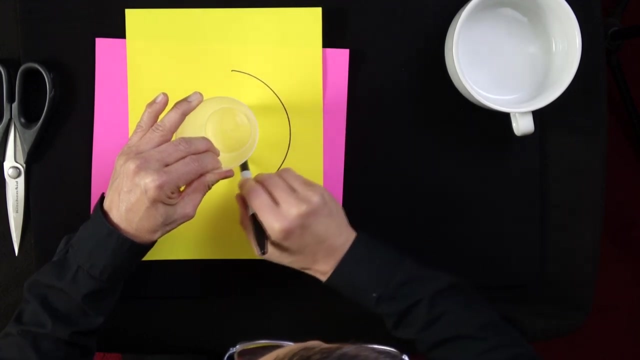 this one. I'm going to use this small diameter here to make an inner diameter. now it's important to try and get this lined up, so so this is at the center here of the outer diameter. so I'm just going to estimate here and let's draw an inner diameter and that's looking pretty good. 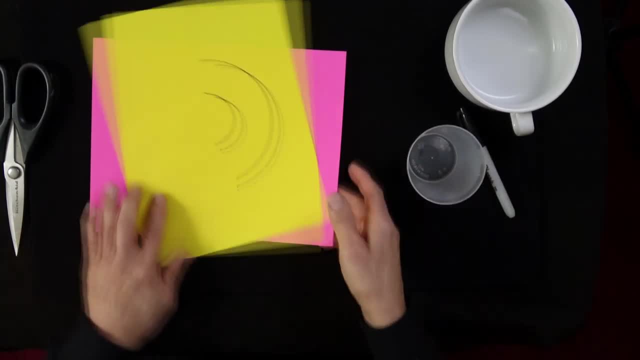 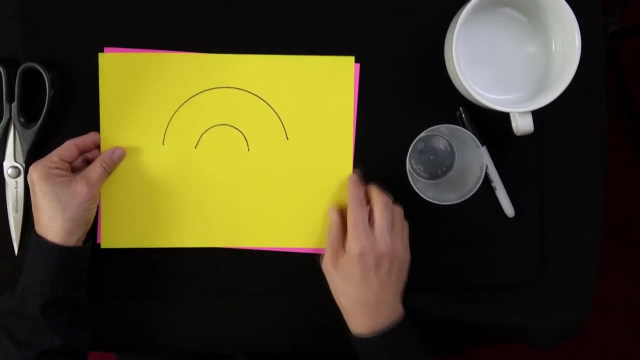 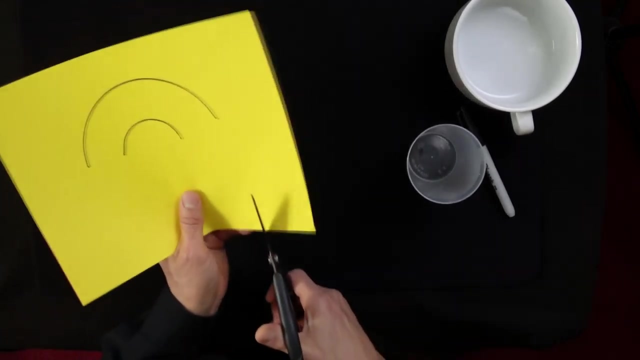 perhaps it's not as even as I would like, but that's okay. for purposes of the trick that will work. so we have an outer diameter semicircle, inner diameter semicircle, line the papers up, and now you're going to use your scissors to cut this out. you want the two papers together because you want these to be. 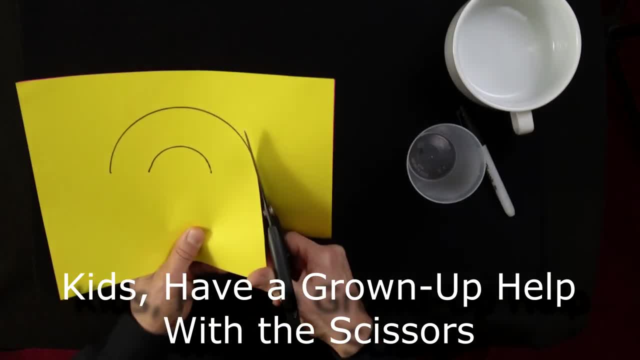 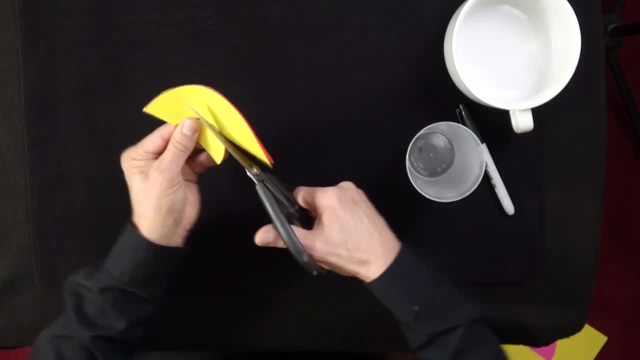 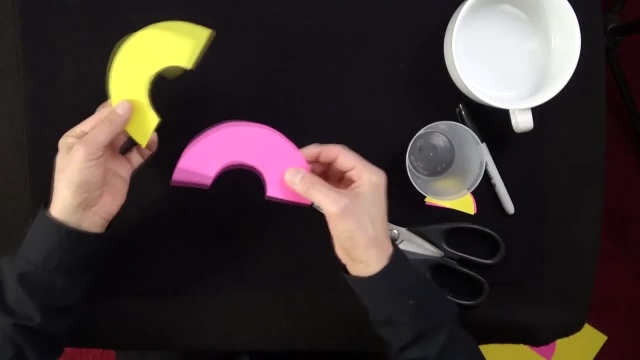 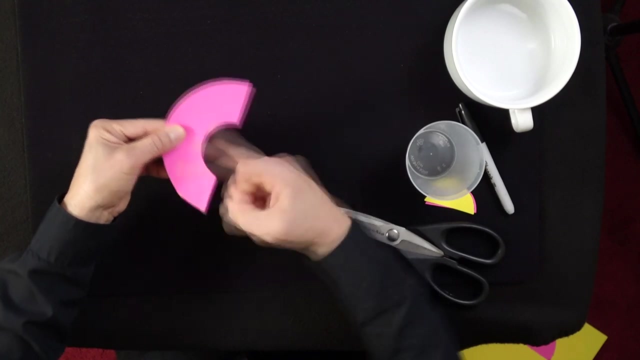 identical, so let's do that. now you have two arcs or rainbows, and the last thing you have to do is you're going to want to trim it somewhere about here so you don't have a semicircle. the trick works a lot better when you 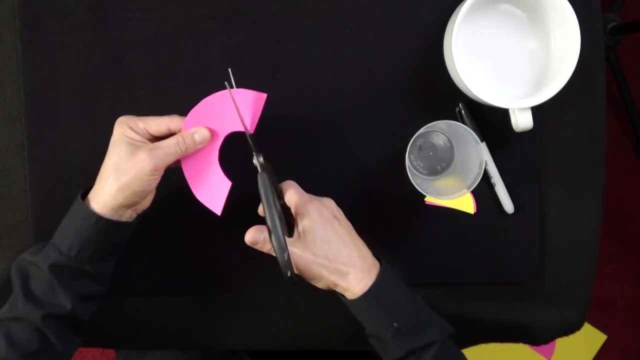 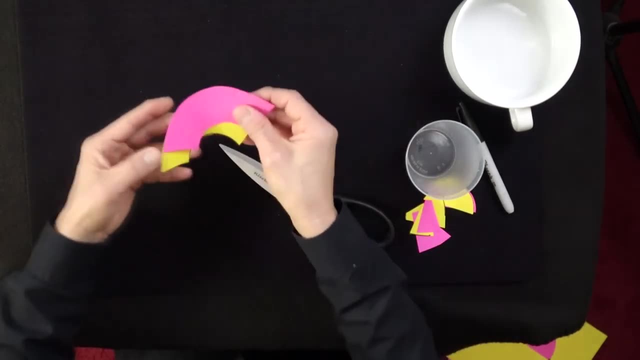 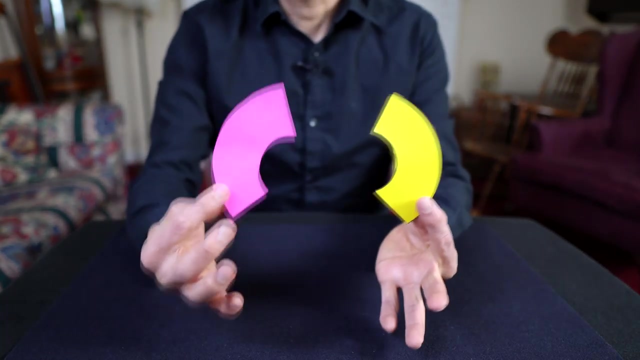 have a shorter Arc, so I'm just going to eyeball that in. I'm going to do something right about there and something right about there. now you have your boomerangs. here's how to perform the trick, as we showed you in the construction. the boomerangs are the exact same size. it's. 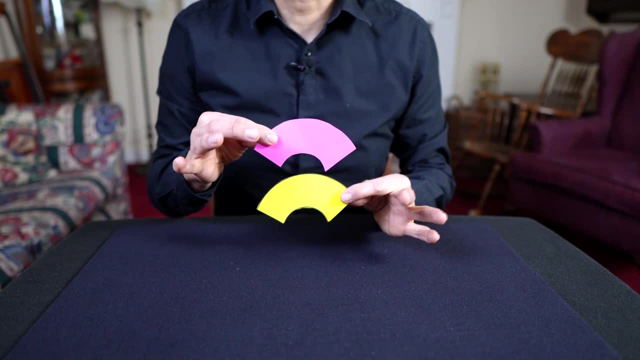 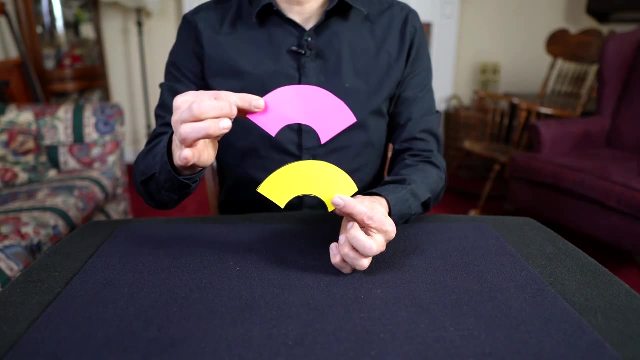 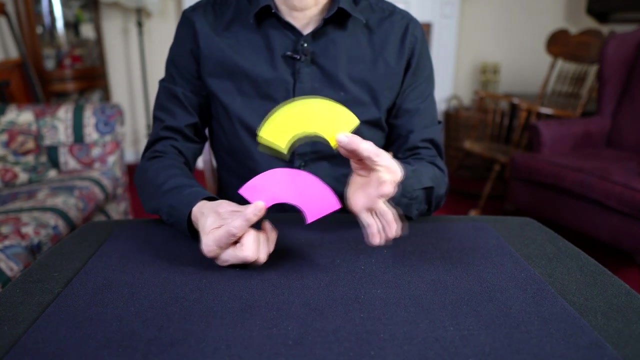 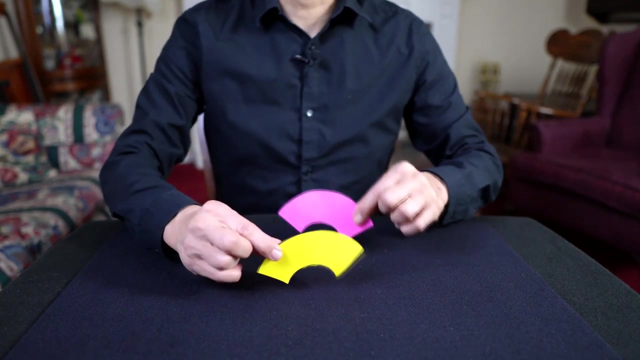 just an optical illusion, turns out that whichever boomerang is held on top always looks smaller. so no matter which way you hold them, the upper boomerang always looks smaller, and that's the secret. so all you have to do is just follow the storyline, just switch. 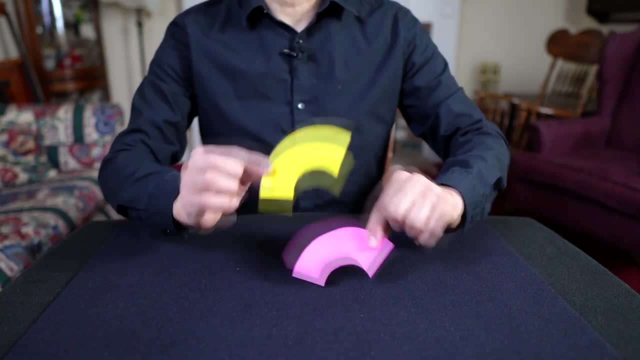 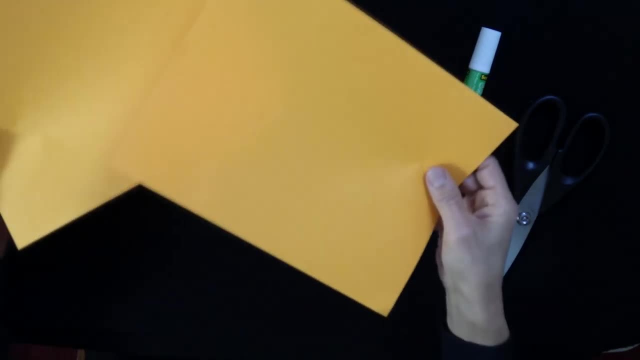 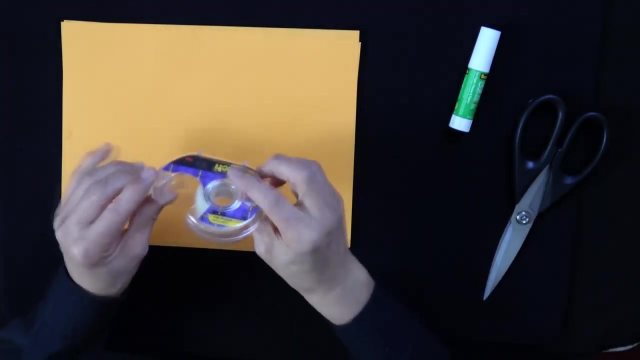 the positions and they'll change- seemingly change in size for spectators. you'll need two sheets of paper same color. of course you can use white printer paper, it's just fine. you'll need some tape. actually the tape is optional, but it really helps and I'll show you a 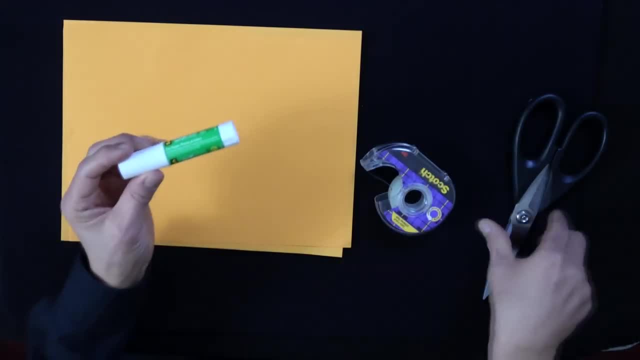 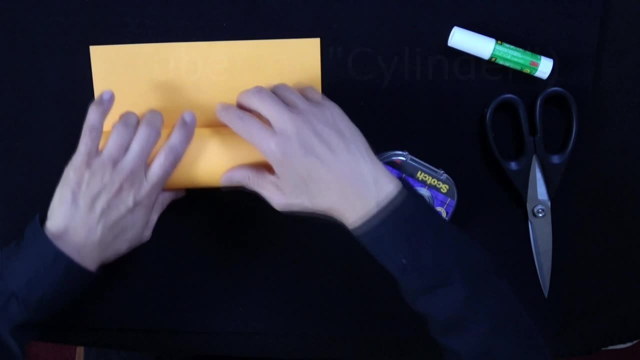 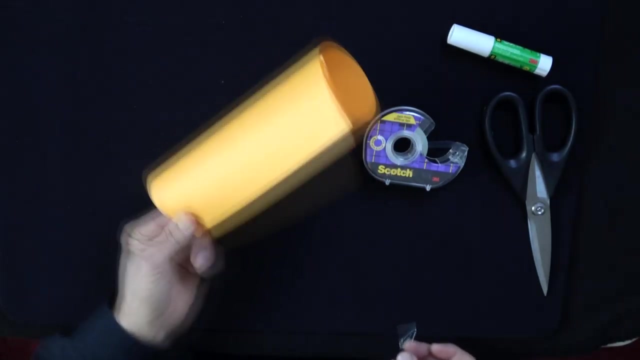 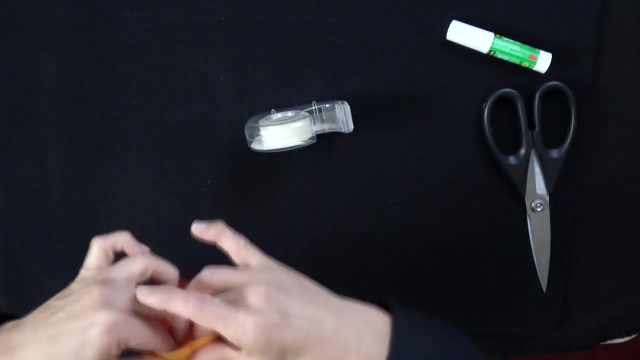 how, why it helps, and you'll need some glue as well as some scissors. so let's get started. first of all, take your first sheet of paper and roll it into a cone, use a piece of tape and, just for good measure, I'm going to put a piece of tape along this seam here. 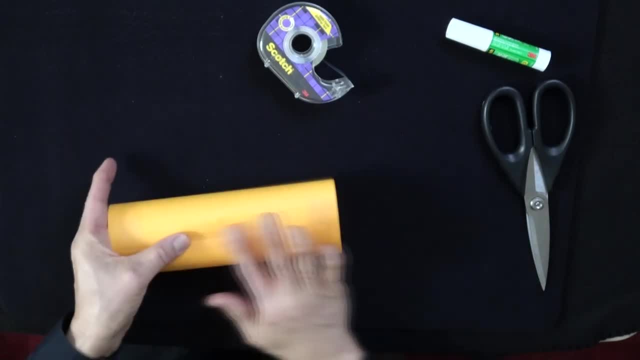 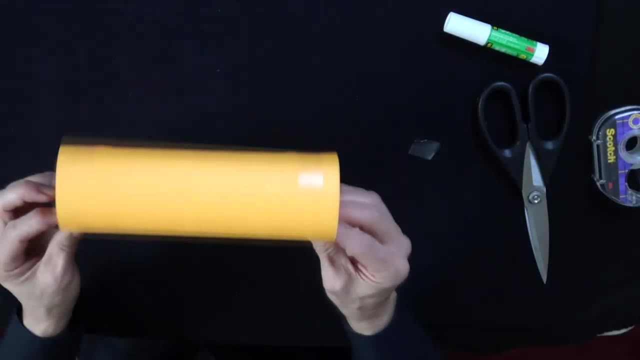 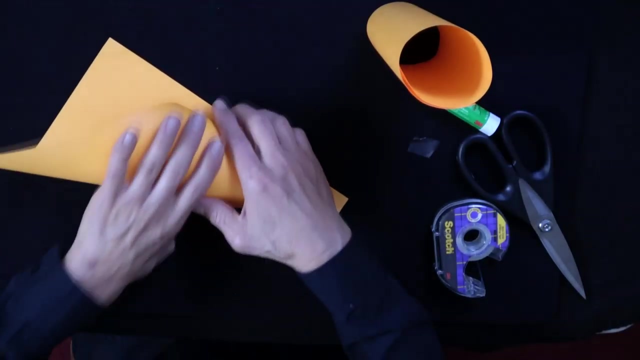 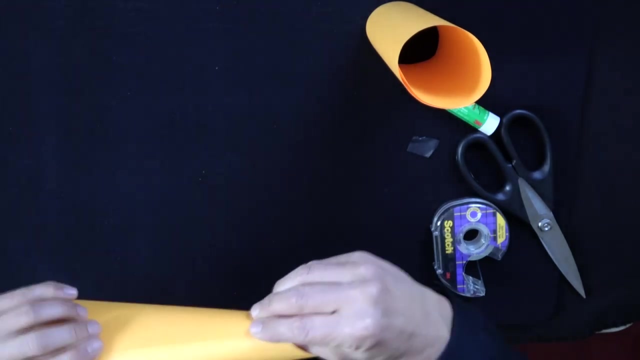 and now I have a fairly nice clean tube second sheet of paper. now this part gets a little tricky. what you're going to do is make something of a cone, but it's not actually a cone. it's going to want a rather small opening here. you might have to experiment a bit. 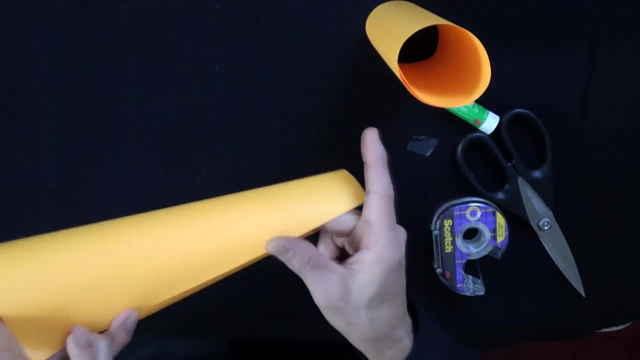 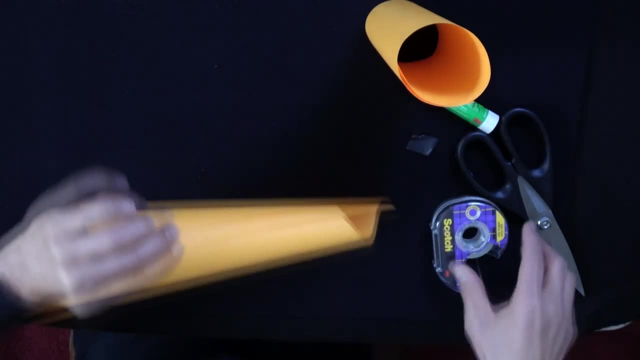 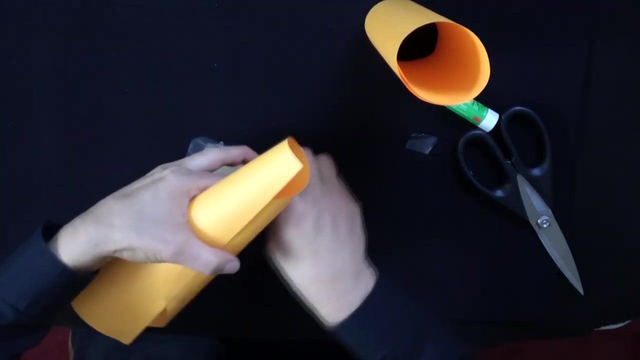 and you're going to want to keep it fairly wide. at the other end you're just making a another cylinder, but it's lopsided. one side is wider than the other. take a piece of tape and hold it there helps to have two pieces of tape on here, because this, uh, admittedly, is a little awkward. 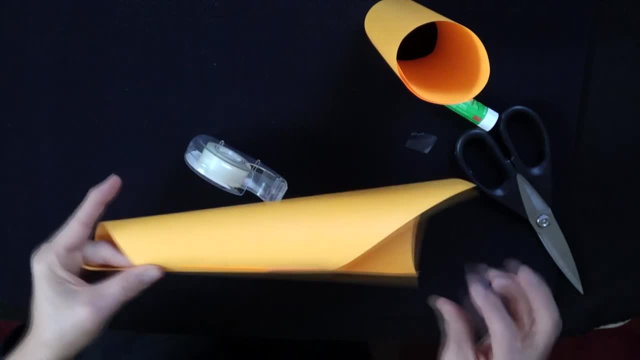 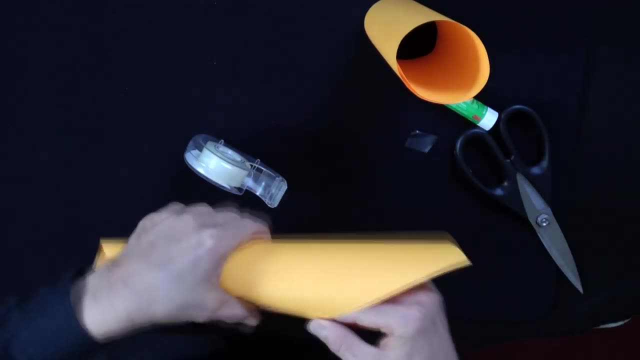 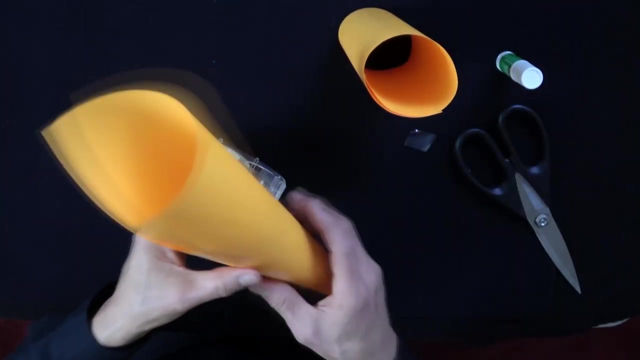 while this trick is great for little kids to perform, it's not an easy one for the kids to put together, so an adult might need to put this one together for the youngsters. we have our regular cylinder over here and we have here a lopsided cylinder. what you're going to do is cut a line. 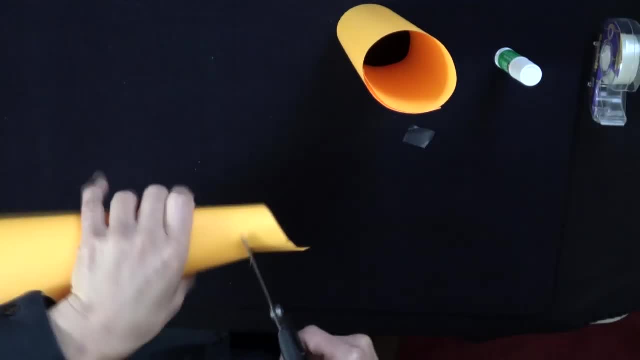 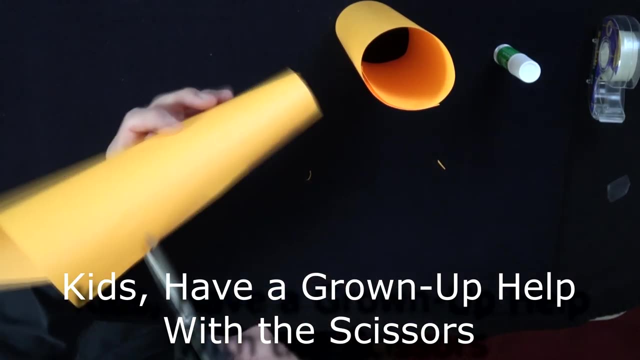 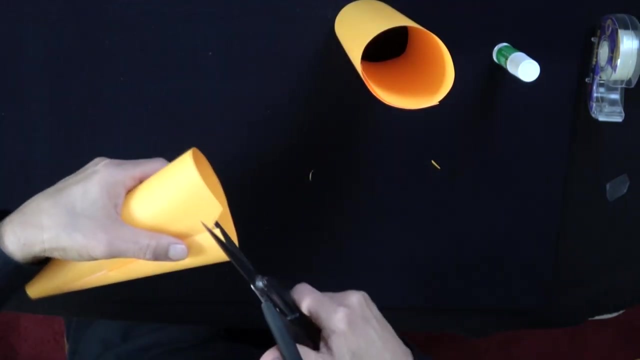 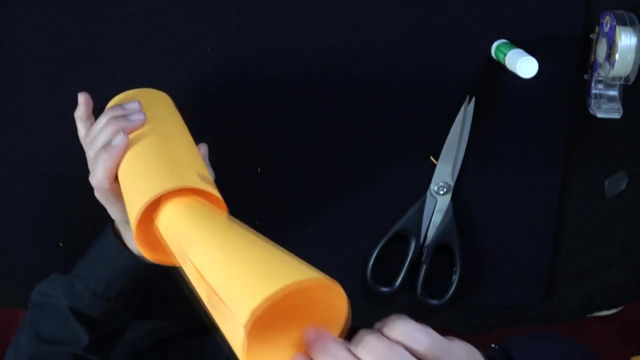 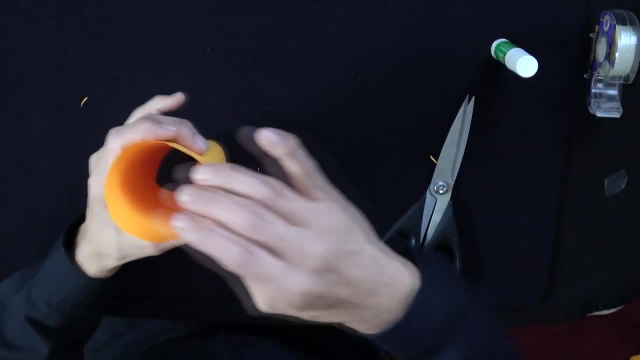 right here. so you want to straighten this out? now take your scissors and do the same thing over here. I now have a cylinder that's slightly lopsided. take this lopsided one and you insert it into the other cone or cylinder there. that's looking pretty good. so what I'm going to do now is I'm 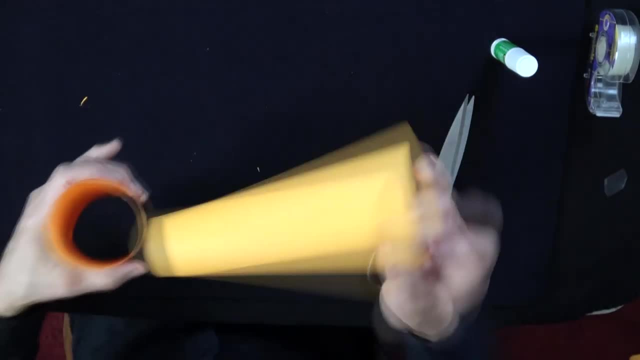 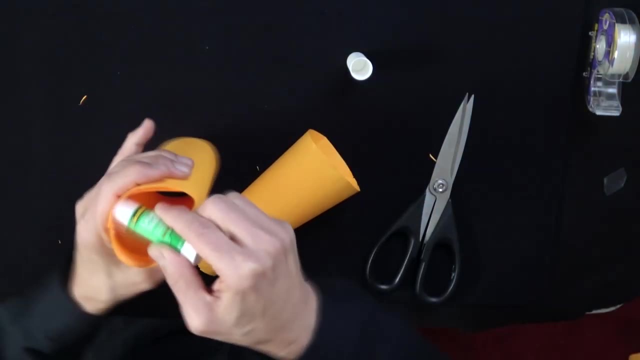 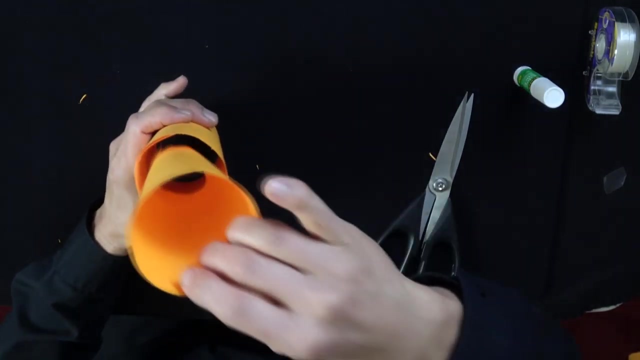 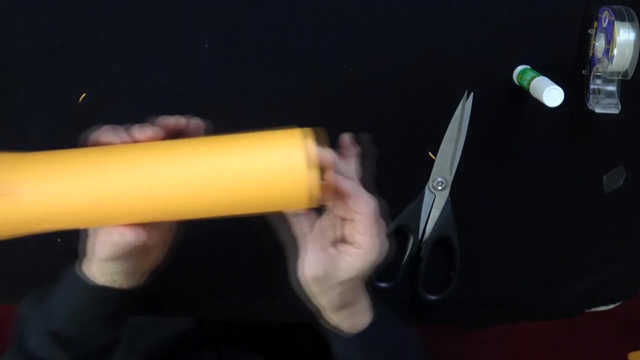 going to put some glue on the inside of here so that will take and hold this right inside here. now take your cone, place it inside so you're adhering this cone to the other cylinder. but if you look from this direction you'll see that there's this cone here. 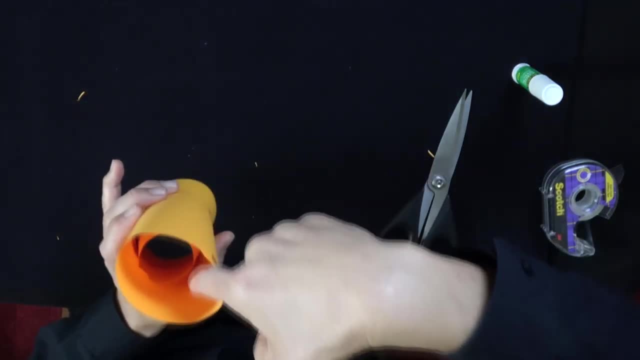 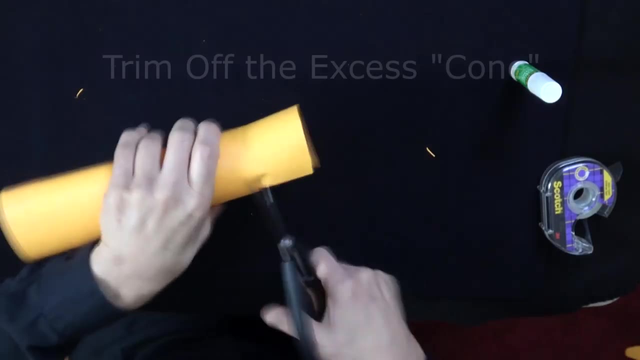 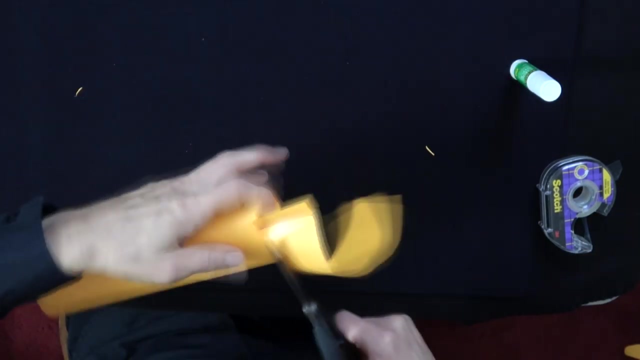 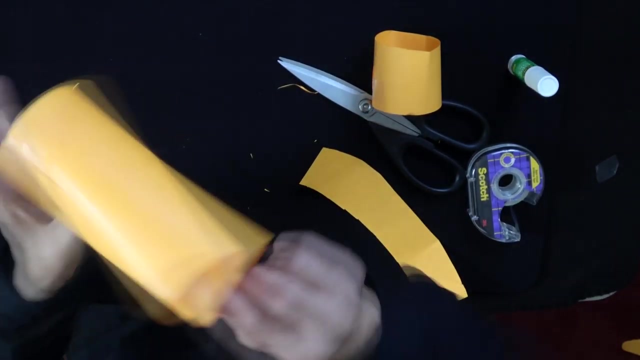 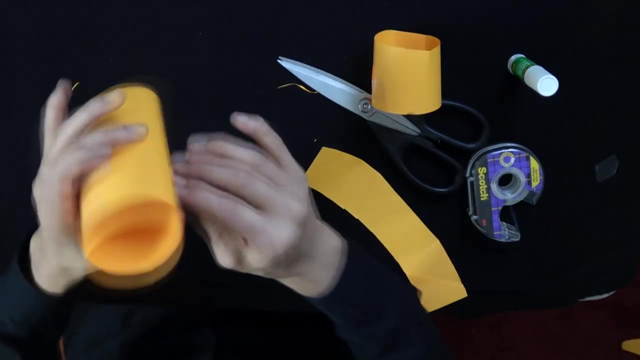 inside and there's actually room on the sides to put things over. on this side it looks fairly normal and there now it's ready to perform the trick. as you can see from this end looks fairly normal. something I would recommend is if you have some different colored tape- color tape here, like maybe. 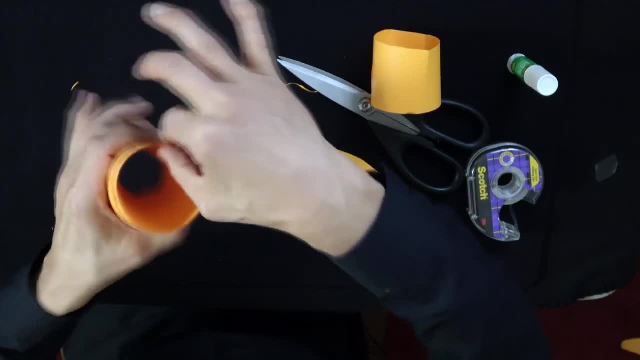 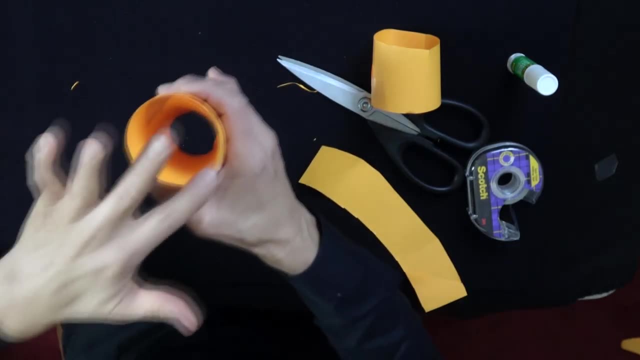 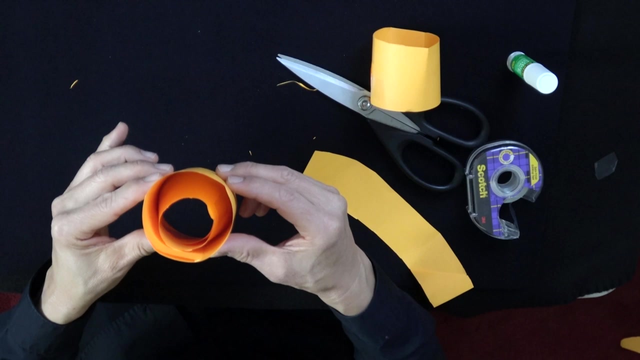 in a red or green or something, you can put it along this edge and kind of seal it up. if you do this close up to people, they might notice that there's a slightly slightly ragged edge here. you can show the tube empty and still have room to hide things.